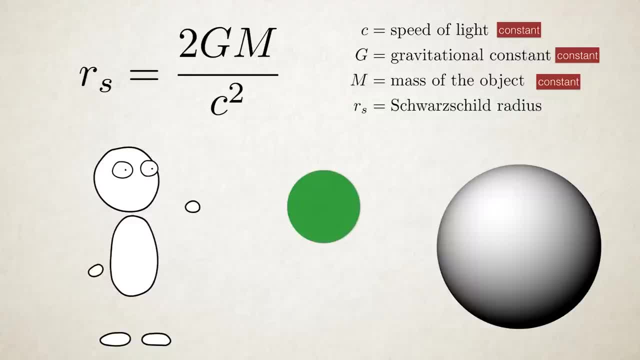 And that's the Schwarzschild radius. It is the radius of a sphere such that if all the mass of an object were to be compressed within that sphere, the escape velocity from the surface of the sphere would be equal the speed of light. This means that in order to escape the gravitational pull of the object, 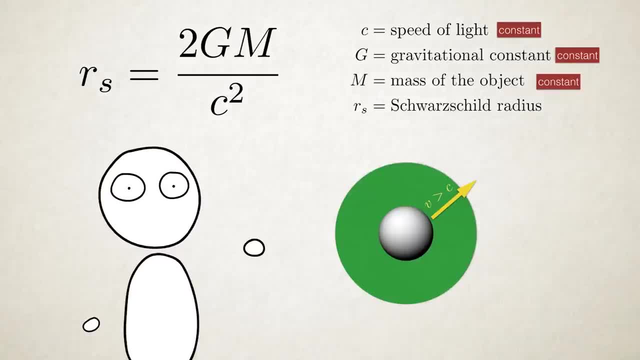 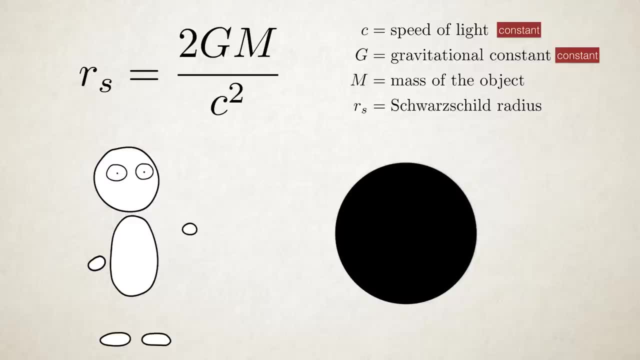 whatever tries to get away from, it would have to move faster than the speed of light. But because the speed of light is constant and nothing can ever go faster, nothing can escape Including light. It's essentially a black pit where anything you put in doesn't come back. 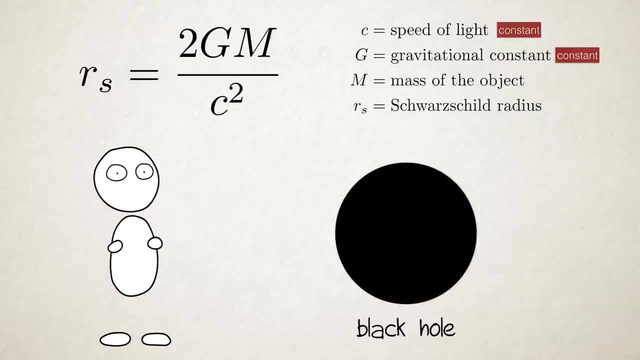 And that's what we call the congressional budget. I mean a black hole, Because the speed of light is such a gargantuan number. its square is fucking ginormous, Which means unless you have an unbelievably big mass, the Schwarzschild radius is very tiny. 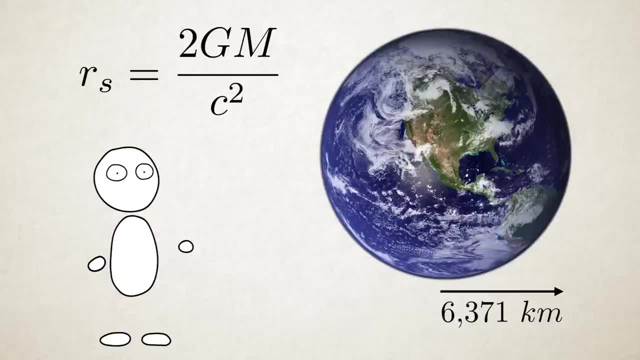 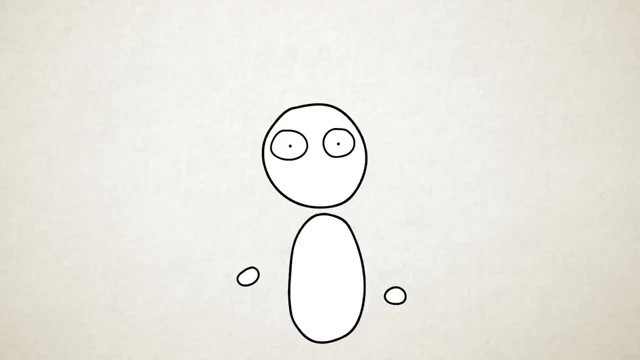 Take the Earth, which is pretty massive. It has a radius of over 6,000 kilometers. Its Schwarzschild radius is only 8 millimeters. I don't think I can even begin to explain the scale of things. It would be like turning this gigantic thing where all of humanity lives cozily. 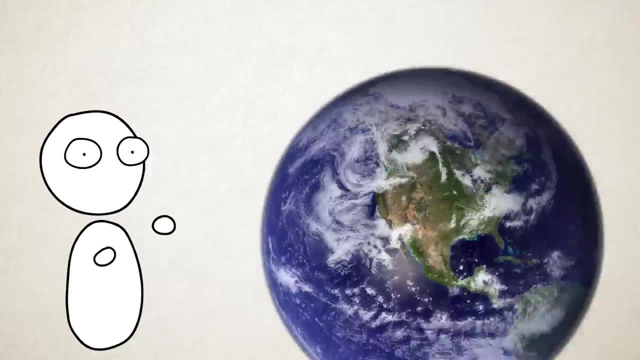 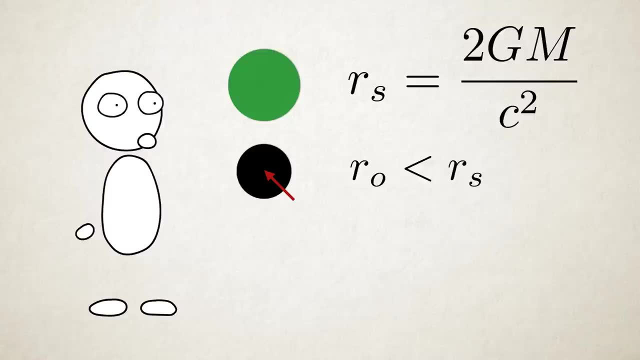 and people take years to travel around by foot into something the size of a penny. Let's go back to the Schwarzschild radius. If the object's radius is less than that, it becomes a black hole. But what happens at the center? 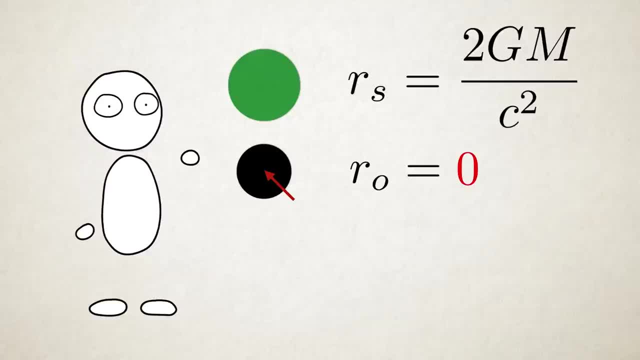 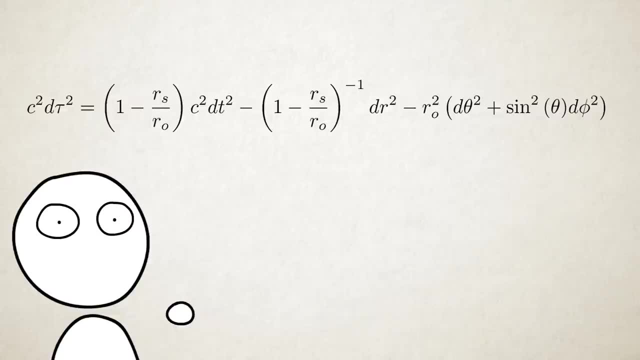 In other words, what happens if the object's radius is zero? This equation defines the shape of spacetime near a spherical mass. Now you don't need to understand all of it, Just have a quick look and see if you can spot the problem. 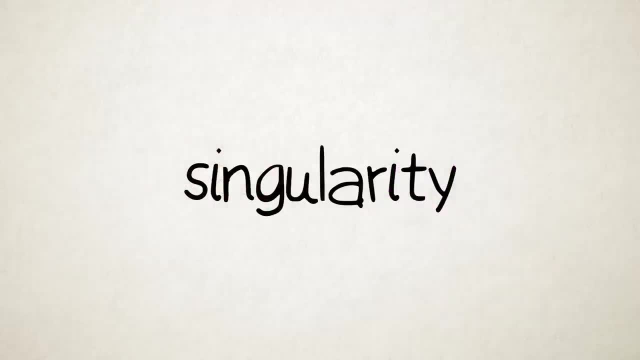 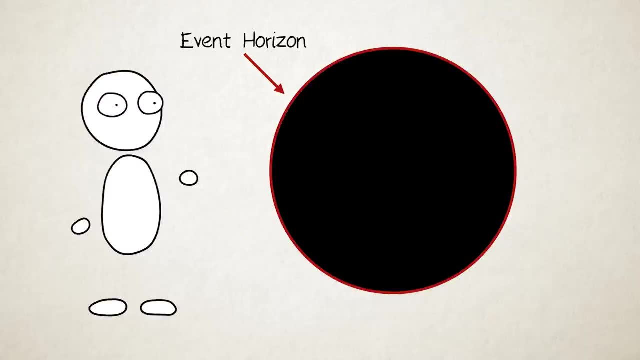 Congratulations. you just broke physics by creating a singularity, An imaginary point in spacetime where all the laws we know don't make any sense. Now let's make something clear. The black hole isn't the singularity, This is the event horizon, sort of a beyond-this-none-shall-return threshold. 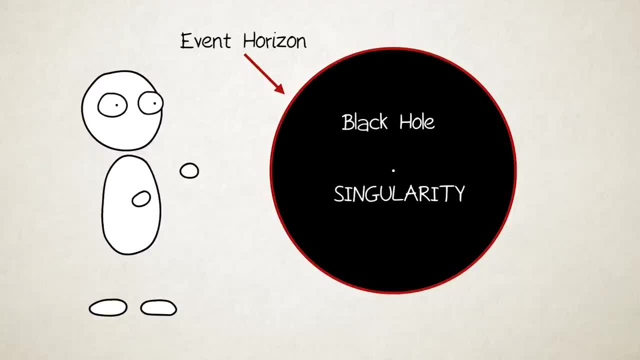 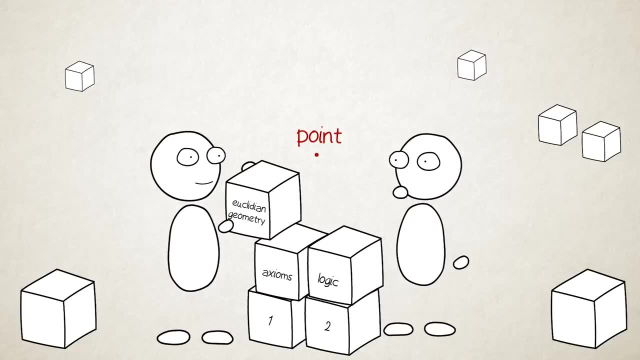 That's the black hole, And in the middle it's where you divide it by zero. The singularity isn't really a place, because in theory it occupies no space and it has infinite density. It's like the concept of point in geometry. It's hypothetical, Except we have experimentally discovered black holes, exactly how Einstein and Schwarzschild have predicted, and there is reason to believe that singularities do exist. There is a copious amount of speculation on what might happen at a singularity, including wormholes, time travel and portals to other universes. 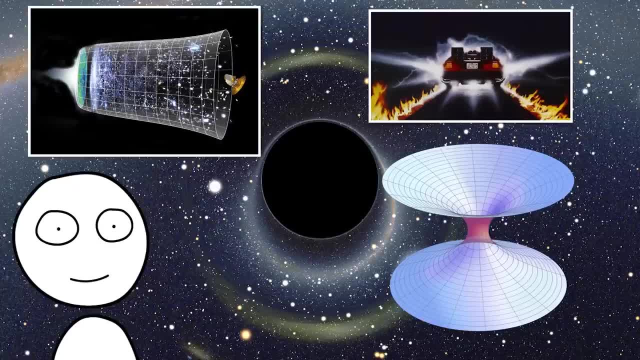 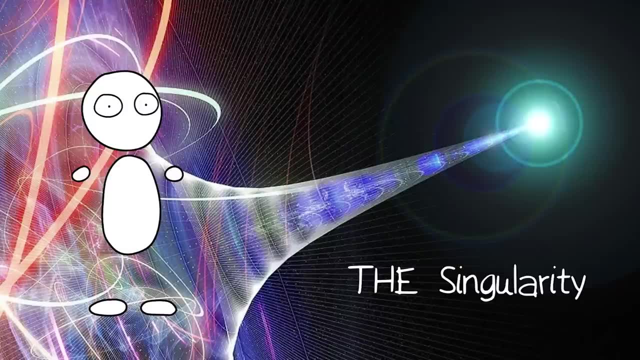 If you're curious about that, please let me know in the comments. We just don't know for sure what happens at a singularity and probably never will, At least not until we get to THE singularity which I'll explain in a later video.